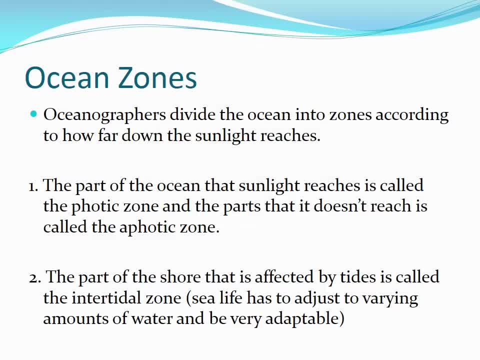 Hi guys, welcome to your lesson on ocean zones. So oceanographers are scientists who study the ocean and they have divided the zone up, or the ocean up, into zones, according to how far down the sunlight reaches. So zones- another word for zones- is sections- So the ocean is divided up. 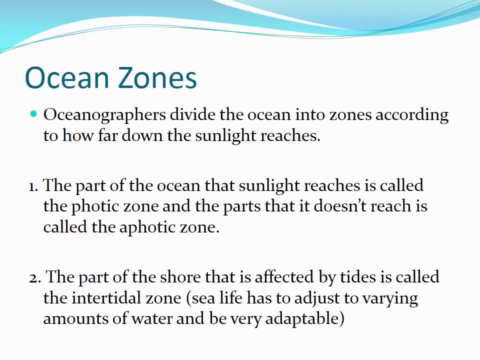 into different sections based on how much sunlight each section gets. So the part of the ocean that sunlight reaches is called the photic zone and the parts that it doesn't reach is called the aphotic zone. So remember, whenever you have the letter a in front of a word, it usually means 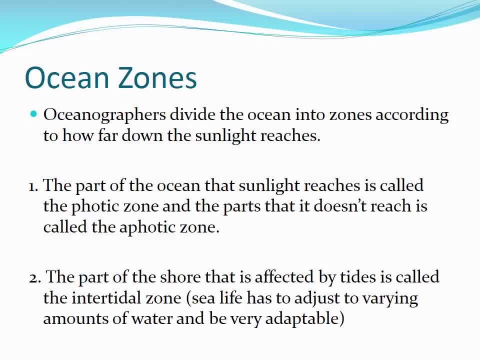 not. So. aphotic means not photic or no light. The part of the shore that is affected by tides is called the intertidal zone. So in this zone, that's where the waves are crashing on the beach and in this zone you have sea life. that has to. 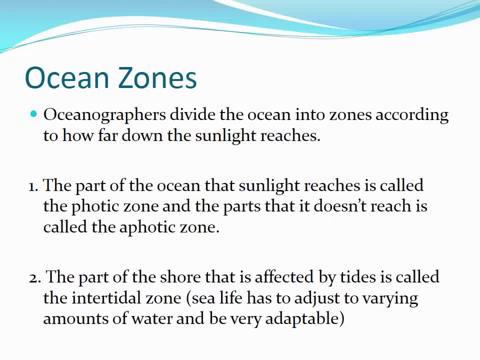 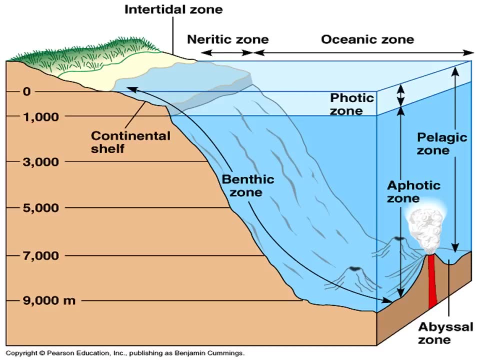 adjust to varying amounts of water and has to be very adaptable. So during high tide the sea life that lives in this zone has to be able to handle more water, and during low tide they have to be able to handle less water. Here's a diagram that kind of breaks down the different zones and so far we've gone over the. 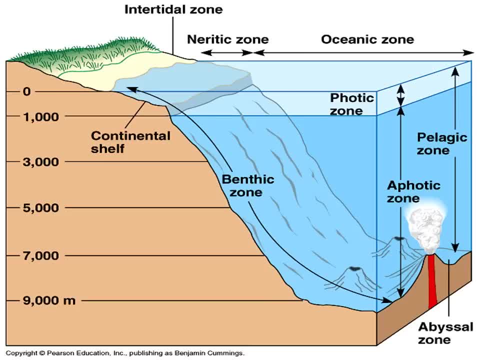 photic and the aphotic and the intertidal. So that's all I want you to focus on right now is at the right hand side, look at the light blue. the skinny top part is the photic zone and then the darker blue. you see the aphotic zone goes from the bottom of the photic all the way down. 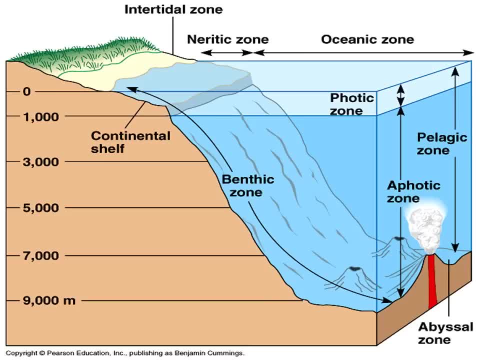 to the bottom of the ocean, to the abyssal zone. So obviously you can see that the aphotic zone is much, much lighter than the aphotic zone. So you can see that the aphotic zone is much, much larger because the ocean is really deep. Sunlight does not reach that far down into the ocean and 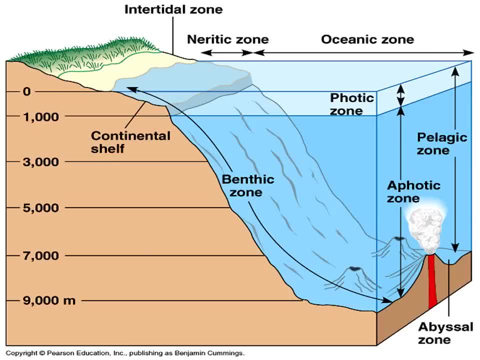 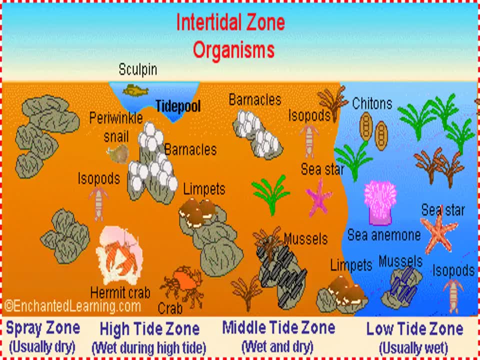 then you can see the intertidal zone that's right on the shore, in the sand, where the waves crash, where the tide comes up and goes back during low tide. These are just some organisms, just a large variety of organisms that live in the intertidal zone. So there's a low tide zone, the middle tide. 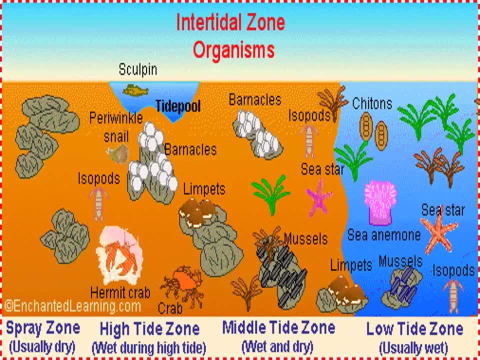 zone, the high tide zone and the spray zone, Which is usually the pretty, pretty dry area. High tide zone is the part that's really really wet during high tide, and middle zone is both wet and dry, depending on what tide it is. So, as you can, 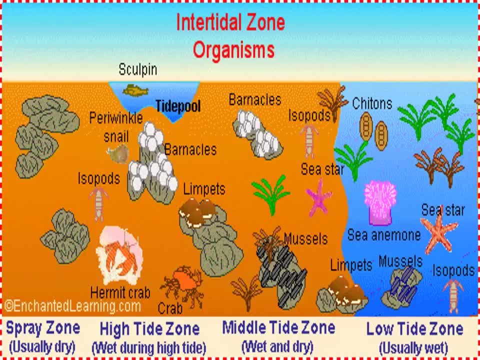 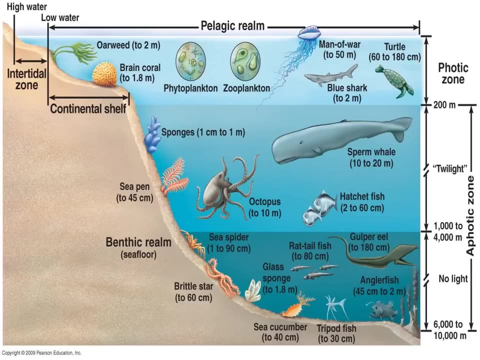 see, there's a really wide variety of different organisms that live in this intertidal zone, and each of them play a very special role in the ecosystem. Here's another diagram for you showing both the photic and the aphotic zone, So you can see what kinds of organisms live in the photic zone. 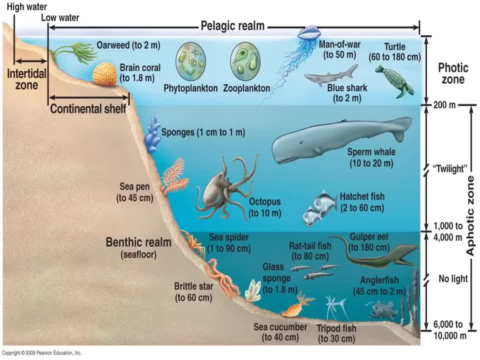 You have sharks, jellyfish, turtles, different kinds of plankton coral, different kinds of plants, and then you see the intertidal zone. You can see where it would be at high tide and where it would be at low tide. So at low tide, that little section in the top left. 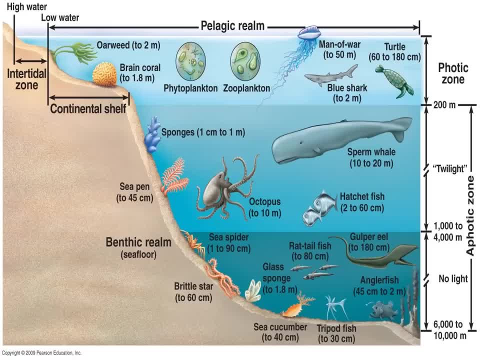 that's covered with water, that says high water. that little section would not have water at low tide. And then look at the aphotic zone. Look at the different kinds of organisms that live there that don't that live where there is not sunlight: Sea cucumbers. those of you who 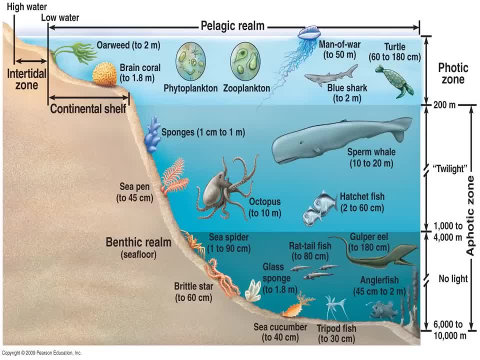 have seen Finding Nemo, Sea cucumbers, the angler fish, that's the fish that that the light comes on, You see that little guy at the bottom right of the screen. Lots of stuff from Finding Nemo in here. Okay, so moving on with the zones. 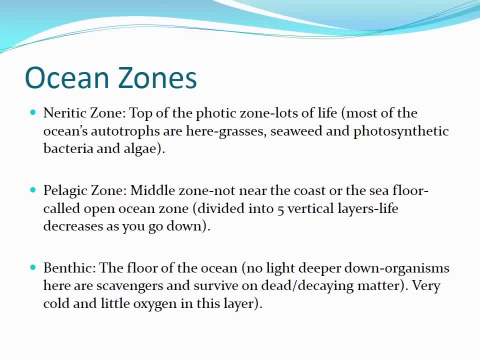 the aphotic zone, the photic zone, and we've done the intertidal zone, so we're moving into more zones. the neuritic zone. the neuritic zone is the very top of the photic zone. lots and lots of life here because there's lots and lots of sea of sunlight. most of the ocean's autotrophs are here. 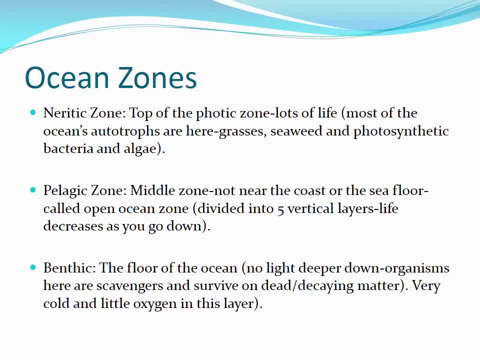 we haven't gotten into ecosystems yet, but when we do, we're going to learn about different kinds of organisms and how they get their food. and autotrophs are organisms that make their own food, and they make their own food from sunlight. so those are grasses, seaweed, photosynthetic bacteria. 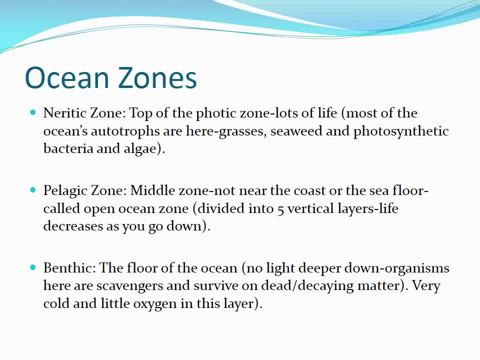 so bacteria that photosynthesize, and algae, lots and lots of of life in the neuritic zone because of the sunlight. the pelagic zone is the middle zone. that's the zone not near the coast or the seafloor and it's called the middle zone. it's the middle zone, it's the middle zone, it's the middle. 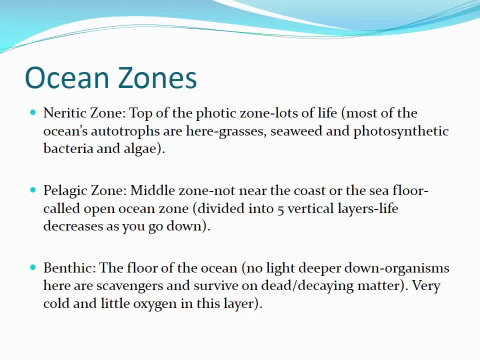 the open ocean zone. it's divided into five vertical layers and as you go down, as you get deeper into the ocean, there's less life and then last is a benthic zone. that's the floor of the ocean. there's no light deeper down and organisms here are scavengers and they survive on dead or decaying matter. it's 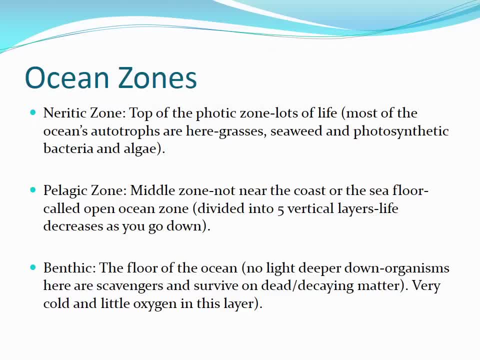 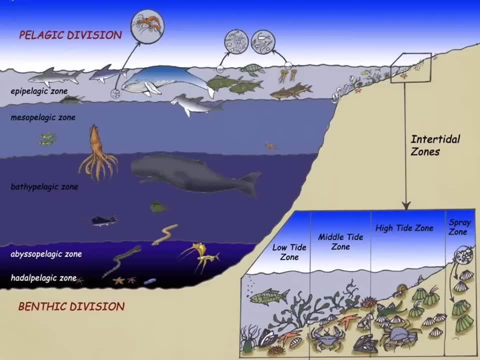 very, very cold down here and there's very little oxygen in this layer, which is why there are organisms that have to survive on things that are dead, all right. so here is another diagram for you. this is showing you the pelagic zone and then the five layers of the pelagic zone. you don't need to memorize those layers. 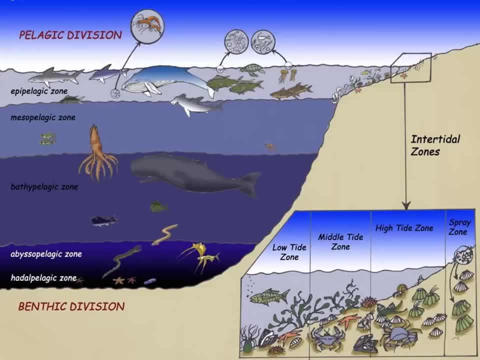 but just understand that as you go down in the ocean there's less life. you can see all the life in the top of the pelagic, the epipelagic. then you go to the mesopelagic and then to the concentric code, the mesopelagic, and if you're 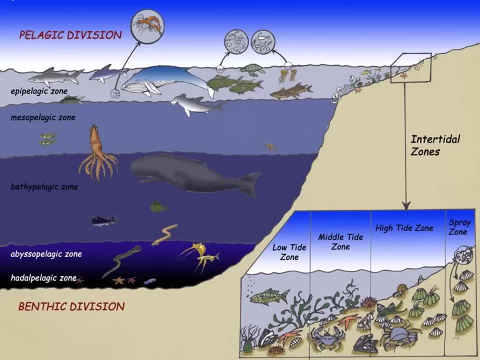 and there's less life- And the bathypelagic- that's where you have the octopus and the whale, And then the abyssopelagic and the hadelpelagic at the very bottom. Another picture off to the right of the intertidal zone. 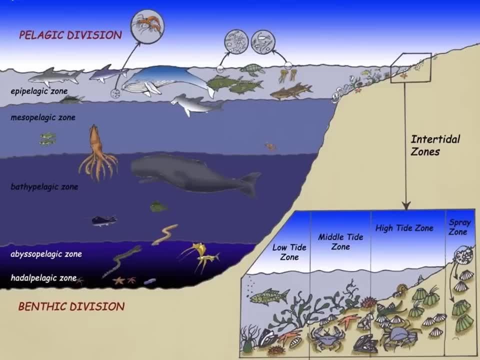 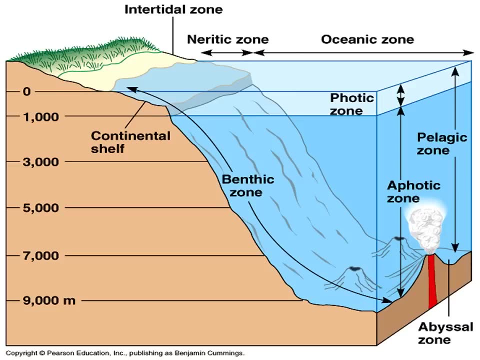 showing you all the different organisms again that live and have to adapt in that zone. Here's that same diagram we looked at in the beginning, only this time we're going to look again. We're going to look at the neuritic zone and we're going to look at the pelagic. 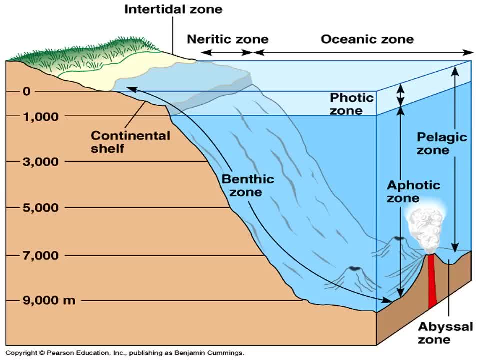 and we're going to look at the benthic. So the neuritic is in the very top. Neuritic is where we had the most life And, again, that's because it has sunlight. That's where all the organisms that depend on photosynthesis live. 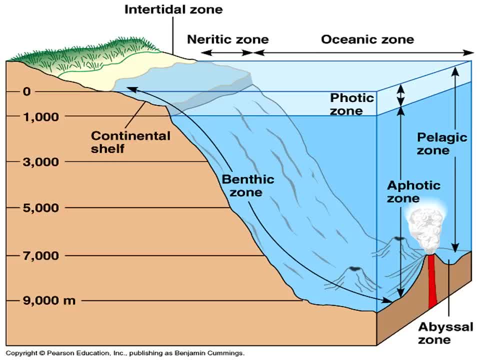 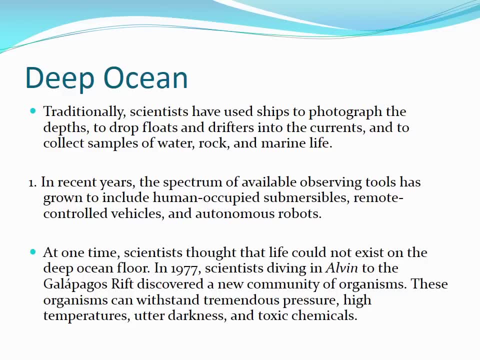 The pelagic is in the middle and the benthic zone is the ocean floor. So deep ocean. Deep ocean is really cool because so much is happening down there, but it's hard to study because it's so far down. So traditionally, scientists have used ships to photograph the 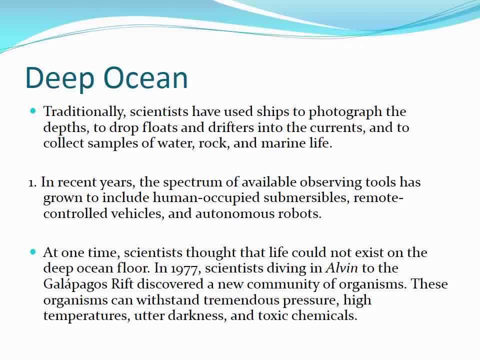 depths of the ocean, to drop floats and drifters into the currents and then collect samples of water, rock and marine life. However, in recent years, the amount of tools for looking at the deep ocean has really grown, and that includes human-occupied submersibles. 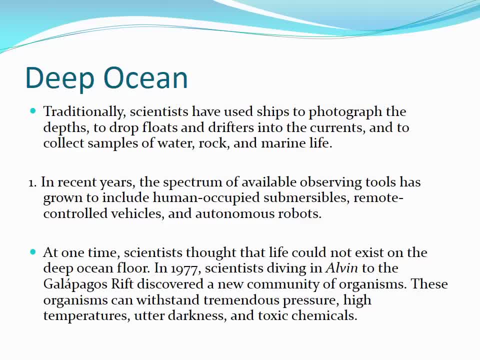 so things that go underwater, that carry humans with them, remote-controlled vehicles and autonomous robots, So robots that can go down to the bottom of the ocean. At one time, scientists thought that life couldn't exist on the deep ocean floor, And in 1977, scientists diving in a ship called the Alvin to the Galapagos Rift. 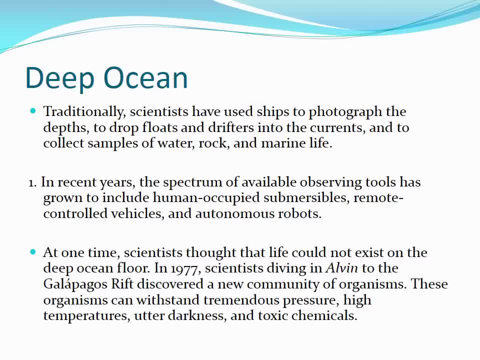 they discovered a new community of organisms Not until 1977. So we think we've known so much about science for so long. But 1977 is not really that long ago, That's just a little bit longer than I've been alive. So these organisms can withstand tremendous pressure Deep down at the bottom of 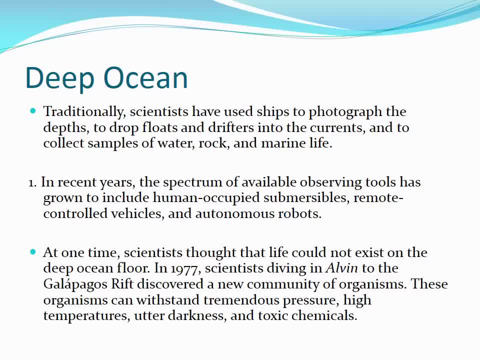 the ocean. there's so much water, so there's high pressure. They can withstand varied temperatures, both high and low temperatures, complete darkness and toxic chemicals. So these organisms that were found at the bottom of the ocean are called albinos, And they're called albinos because they're 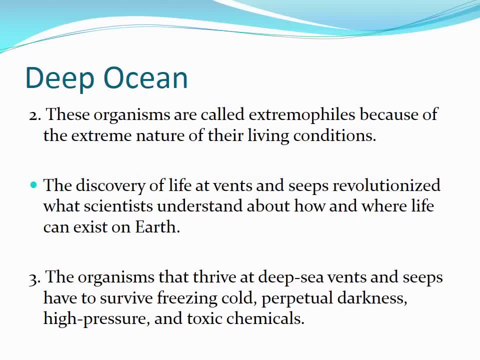 called extremophiles, And they're called extremophiles because they live in extreme living conditions. The discovery of life at these vents and seeps revolutionized what scientists understand about how and where life can exist on Earth, So the organisms that thrive at deep sea. 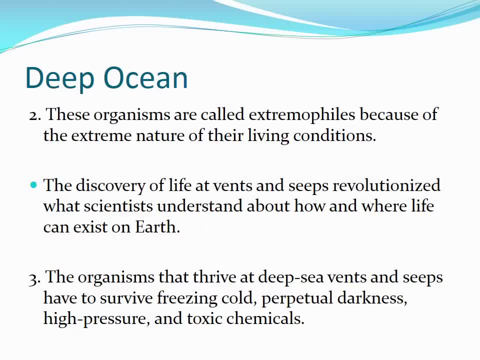 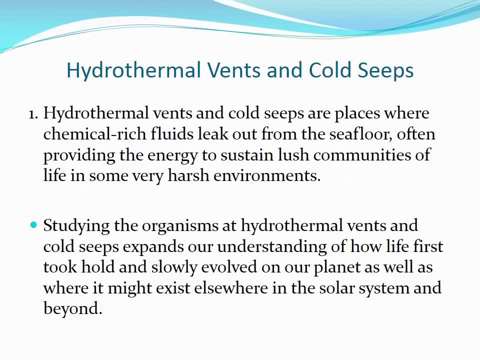 vents and seeps have to survive freezing, cold temperatures, total darkness, high high pressure and very, very toxic chemicals. So the organisms that thrive at deep sea vents and seeps are called hydrothermal vents and cold seeps And, as you can see from the word hydrothermal you have the word prefix hydro, which 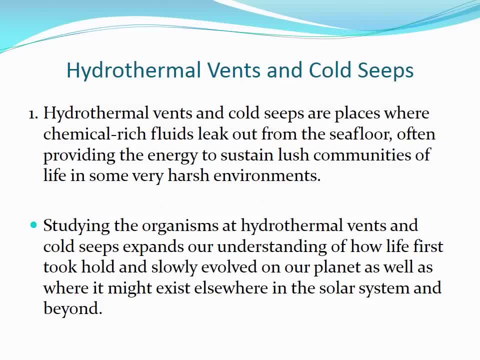 means water, and thermal, which means heat. So you have hot water and then you also have something that's really really cold. So organisms either live in the really really hot or the really really really cold. So hydrothermal vents and cold seeps are places. 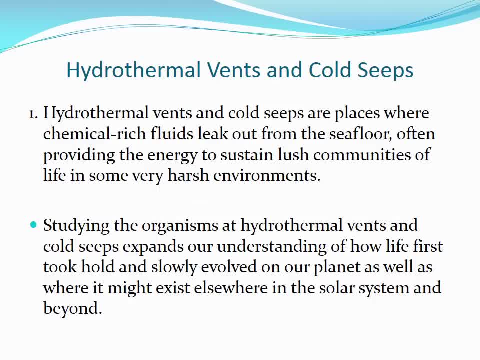 where chemical-rich fluids leak out from the sea floor, often providing the energy to sustain lush communities of life in very harsh living environments. So the fluids that are leaking from the sea floor bring really, really large amounts of chemicals, And those chemicals are actually 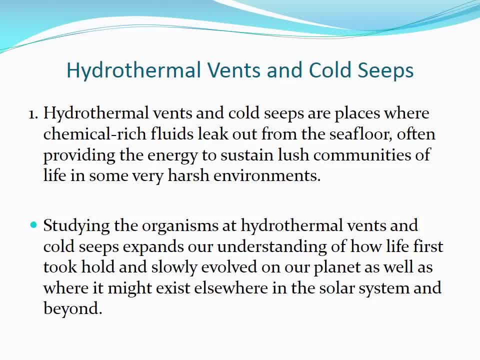 what keep those organisms alive. So studying the organisms at hydrothermal vents and cold seeps really expands our understanding of how life first took hold and slowly evolved on our planet, as well as where it might exist elsewhere in the solar system and beyond. So these organisms that live, 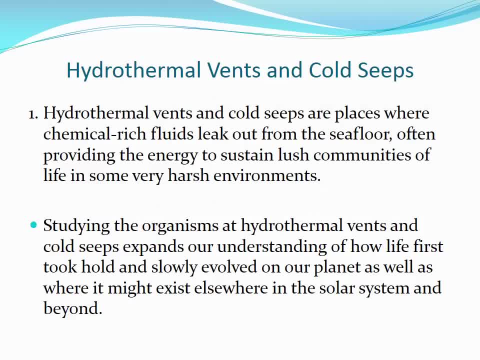 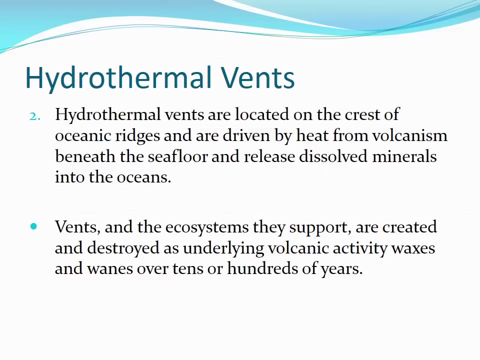 down in these harsh environments are the same kinds of organisms that came to be when life first started on Earth, And so by studying these, scientists can really really understand, or at least try to understand, how life has evolved on our planet. So hydrothermal vents are located on the crest or the top of oceanic ridges and are driven by heat. 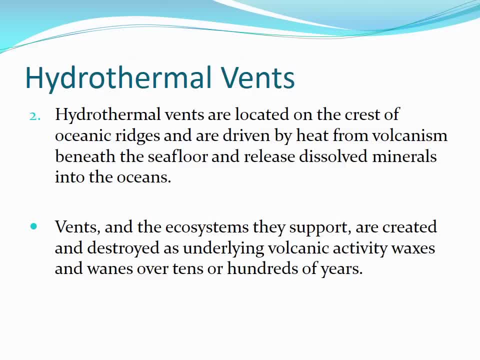 from volcanism beneath the ocean floor. So that's where that heat comes from. is volcanoes under the ocean floor And they release dissolved minerals into the ocean Vents and the ecosystems they support are created and destroyed as the volcanoes get worse and less over time. So when you have lots, 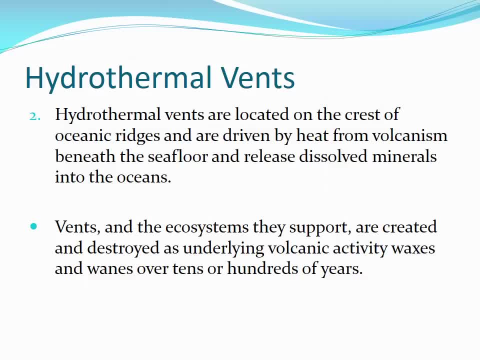 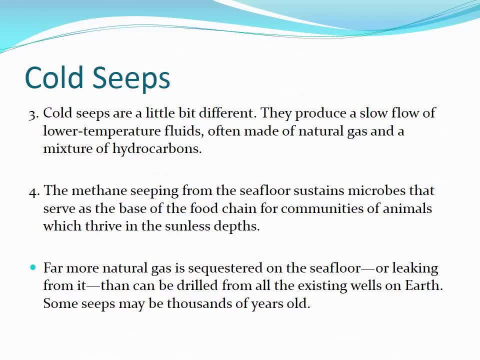 of volcanism underneath the ocean floor, those vents and those ecosystems might be destroyed. When you have very quiet volcanic activity, then the vents and the ecosystems can live All right. so finishing up cold seeps. They're just a little bit different. They produce a slow, 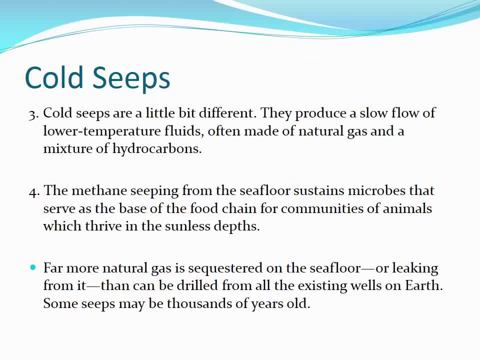 flow of low temperature fluids, and they're often made of natural gas and a mix of what are called hydrocarbons, The methane, which is a form of gas seeping from the sea floor. that is actually what sustains microbes And microbes. we're going to get into microbes and 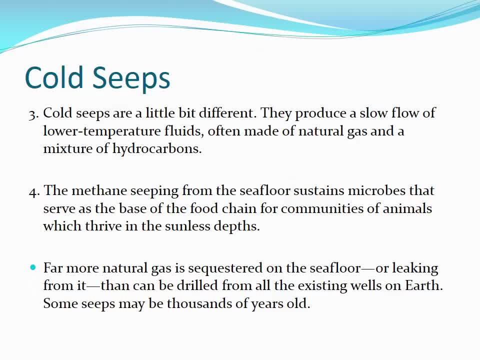 diseases in our next unit, but they're a very, very, very tiny form of life, And microbes serve as the base of the food chain for communities of animals that live down in this zone, where there's no sun and it's really cold. So far more natural gas is sequestered from the on the sea floor. 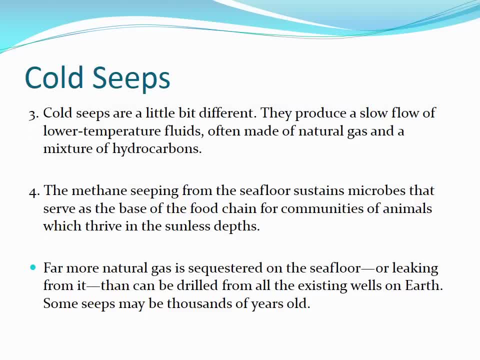 or leaking from the sea floor. So far more natural gas is sequestered from the on the sea floor or leaking from it Than can be drilled from all of the existing wells on earth. Some seeps in the ocean may be thousands of years old, So we have these cold seeps where we have natural gas leaking. 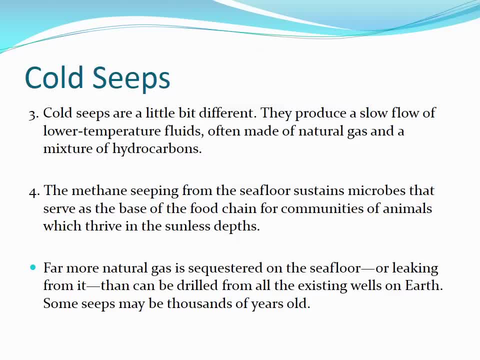 Okay, so natural gas, gas isn't always hot. In this case, natural gas leaking out is very cold, And these different microbes, these tiny, tiny, tiny forms of life, are able to survive and become the base of the food chain for many communities of animals that that live on the sea floor. 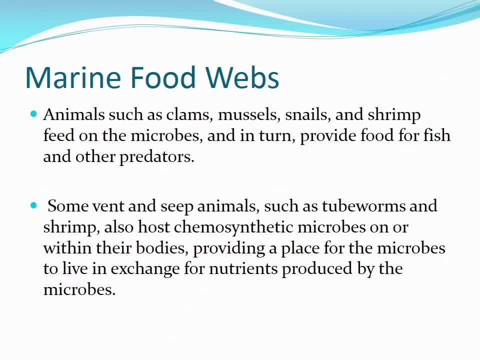 Okay, so the better consensus here is that they live off of microbes and not look properly. So whether they make a living because, like poisonous Copic, or they let academics live off the microbes And that could be someone alive, somebody that's not a human. Others who are. 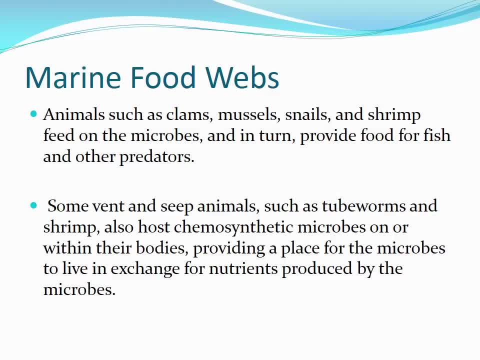 human and otherwise, acabarly, and like most people who don't actually be called institutes. Okay, so animal, you get it. It can be unaffilahmed, full, you know, in that combo, andopoliticized. The idea is that we have ynes and usin and ovals. They're both a. branch of the animal and they also do an interest inulo drogangen consumed by people around us. So animals such as clams, mussels, snails, shrimp- they feed on those microbes And in town they provide food for fish and other predators. 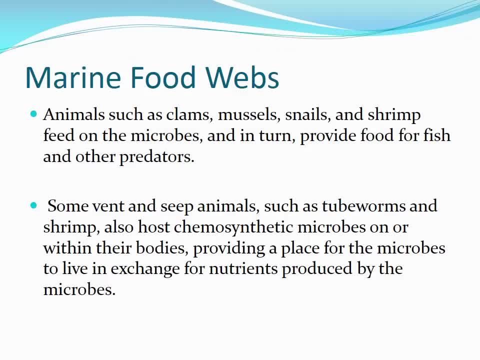 So we have photosynthetic, which are animals or organisms that depend on light in the sun, from the sun, and chemosynthetic, which are animals that depend on chemicals, and these are chemicals from the ocean. So some of these animals host chemosynthetic microbes on or within their bodies, providing 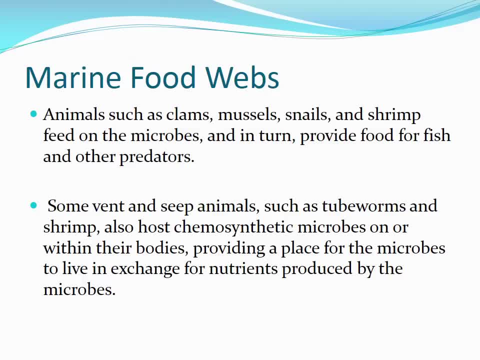 a place for the microbes to live. In exchange, the microbes give them nutrients. And again, we haven't gotten into ecosystems yet, but we are going to get into the types of symbiotic relationships and we'll be getting into food chains and food webs and